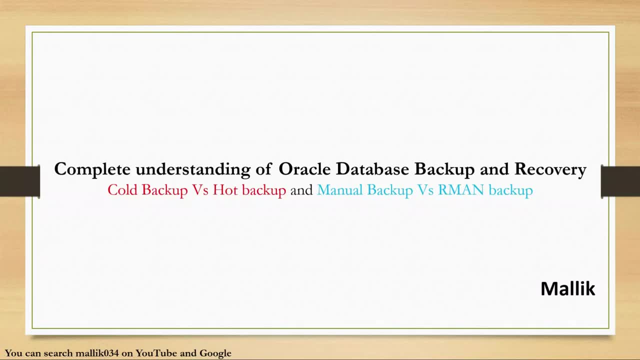 Hello everyone, welcome to malik034 channel. This is Malik Arjun. In this today's session I'm going to explain about complete understanding of Oracle database backup and recovery: What is cold backup and what is hot backup, What is manual backup, What is RMAN backup, What are the difference between these different kinds of backups And what is a consistent backup and what is inconsistent backup, And when we do incomplete recovery and when we do complete recovery. everything I'm going to explain in this today's session. I'm damn sure after this today's session I'm going to be able to explain everything. 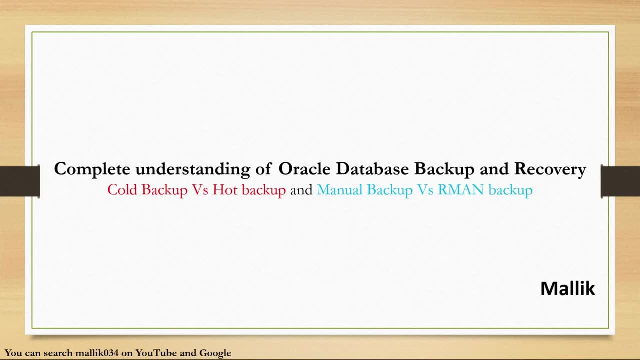 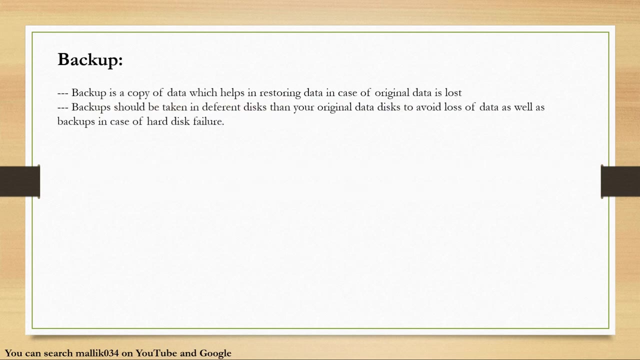 In this today's session, everyone will feel that backup and recovery is not that challenging. It is so simple. First of all, if you are new to my channel, I request you to go back to YouTube and search for malik034 and then please do subscribe. If you like my video, please share, like and comment. Getting started with today's session: Backup. Backup is a copy of data which helps in restoring data in case of original data is lost. Backup should be taken in a different disk than your original disk. To avoid lost data, you should take backup in a different disk than your original disk. 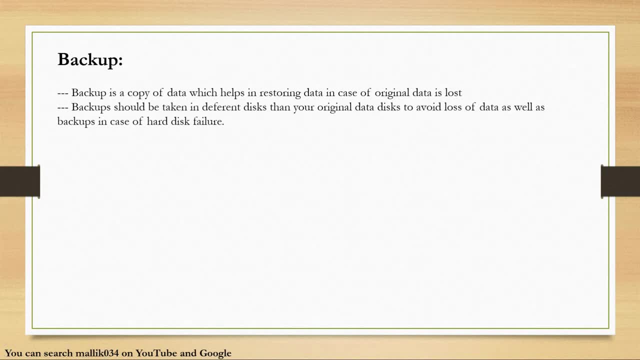 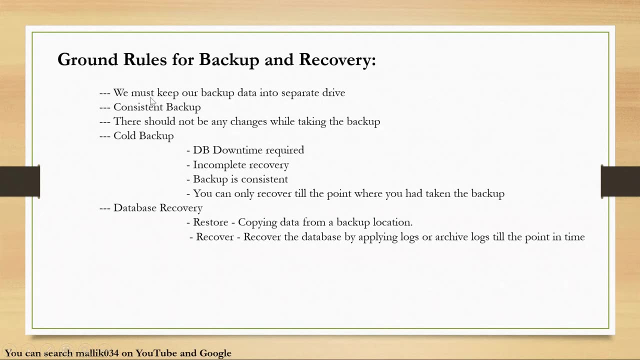 Because of both your original data and backup data in case of disk failure. That is precisely a backup, And what are the ground rules for the backup and recovery? We must keep our backup. you know backup data into separate drives right And backup should be consistent. There should not be any changes while taking the backup And the cold backup. precisely, cold backup is requires a DB downtime and it is incomplete. recovery and backup is consistent. 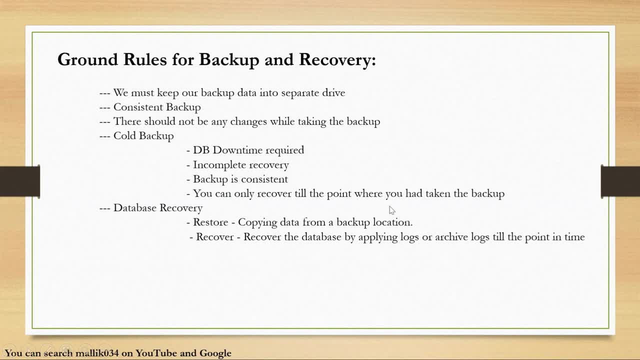 And you can only recover till the point where you have taken the backup. After that, if any changes, you cannot be able to restore it. in case of cold backup And database recovery: What is database recovery? It has two parts: One is a restore and one is a recover. Restore is a copying data from you know backup location to your original location And recover, recovering like recovery. Recovery is the recovery, the database, by applying all the logs and archival. 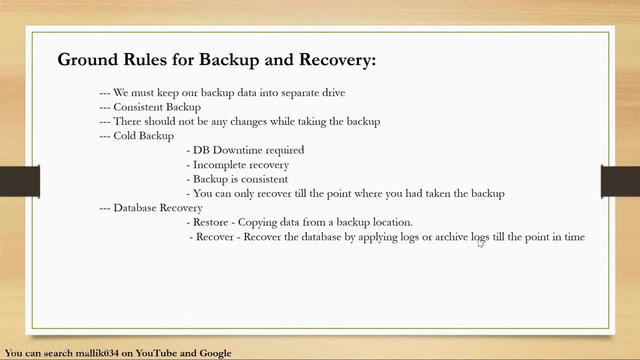 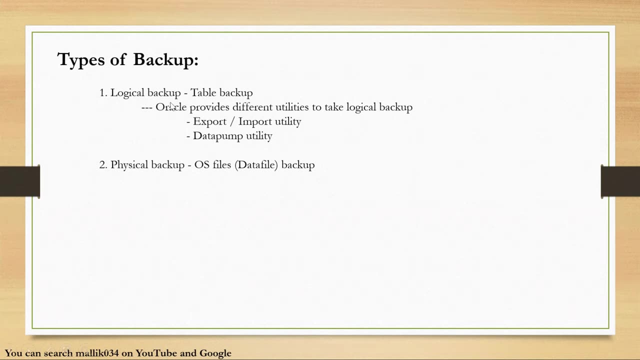 logs till the point in time, till the point in time recovery. These are the you know, basically ground rules for any backup and recovery. And what are the types of backup? you can see There are logical backups or physical backups. Logical backups are table backups or schema backups or you know anything, any view or whatever backup. Oracle provides the different utilities to take logical backups, like export or import or data pump utilities. 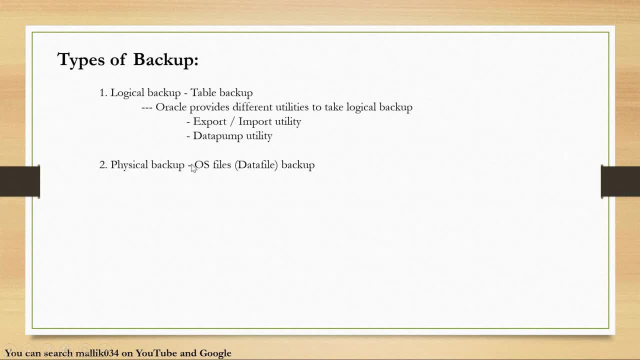 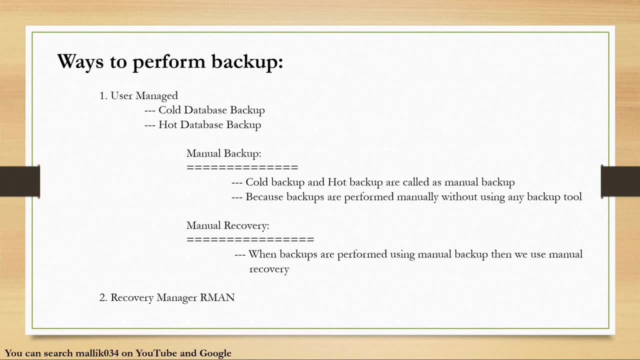 And for the physical backup is nothing, but you know copying or you know backing up your OS data files. Those are the physical backups And ways to perform the backups. how you can perform your backup- like there is a manual user managed or recovery managed or man The manual user managed- are like a cold database backup or hot backup. You know, in cold backup is nothing but you're shutting down your database and manually copying your database. 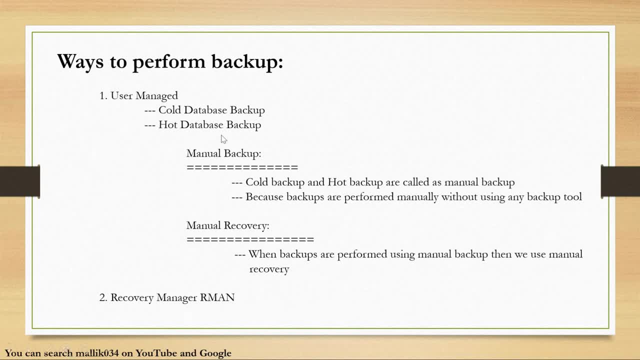 You're using OS command and then taking the backup And in case of hot backup, like inside hot backup, I can say manual backup and manual recovery. What is that manual backup and manual recovery? The cold backup and hot backups are called manual backups. Why we call it a manual backup? Because backups are performed manually using any backup tool. Right Without any backup tool. Manually we can copy like CP In cold backup we will shut down the database. 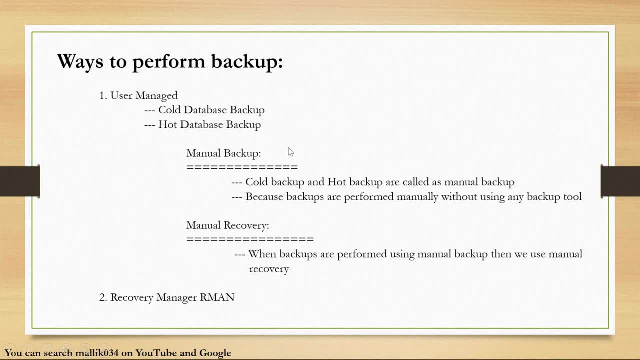 We'll just CP using OS command, CP, and then copy all the data files and control files And in case of hot backup, we'll put database into begin backup mode and then manually we can copy all the data files and control files, everything. And we're not going to use any backup tool. All is going to be OS command, like CP command, And manual recovery. when backups are performed using a manual backup, like either cold backup or hot backup, we use a manual recovery And the other tool is a recovery manager, RMAN. RMAN is a recovery manager. 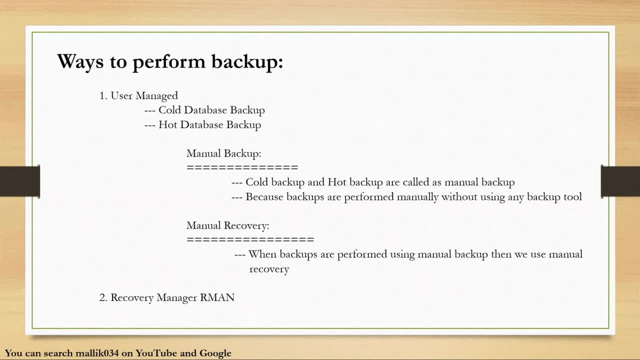 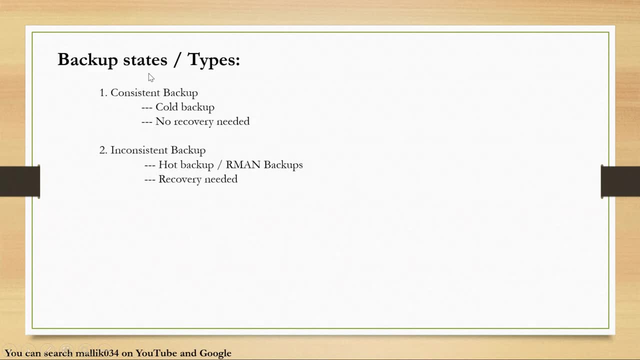 RMAN is a backup tool and recovery tool. We can do perform or backup and recovery using this RMAN And backup. you know states or types, backup types or backup states. I can say the consistent backup or inconsistent backup. Consistent backup or like cold backup and no recovery needed, And inconsistency backups or like hot backups or RMAN backups, where the recovery is needed. And coming to the recovery, what is recovery Like? what are the type of recovery? Recovery is a recovery manager. 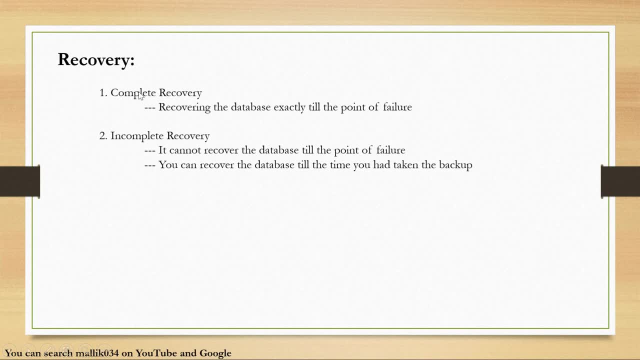 I can say that restoring your database and applying the logs or archives on top of your- you know- restored database. So there are two types of recovery, like complete recovery and incomplete recovery. The complete recovery is like recovery the database exactly till the point of failure, And incomplete recovery it cannot be recover the database till the point of failure. You can recover the database till the point you had taken the backup, Or after that you can apply the recovery manager. 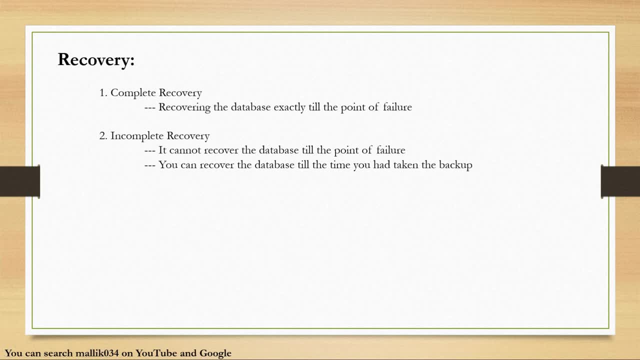 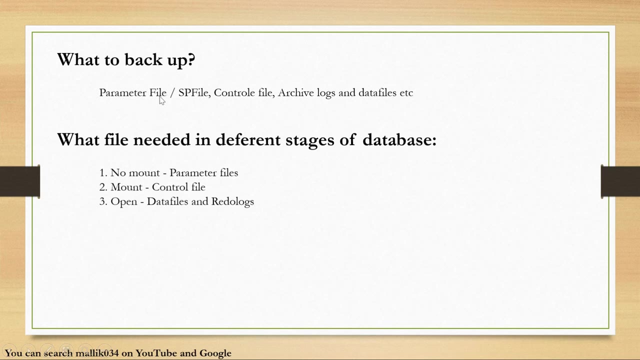 Or after that you can apply the archive logs till whatever the time it is available. Where in this, in case of incomplete recovery, there might be a slight loss of data, And in complete recovery, there is no data loss. And what to backup? The next question comes: what to backup? You have to backup your P file, SP file, control file, archive logs and data file. You know whatever you, you know desire to keep it secure, And then you know whichever files is needed for your restoring purpose And what files to be, you know, restored. 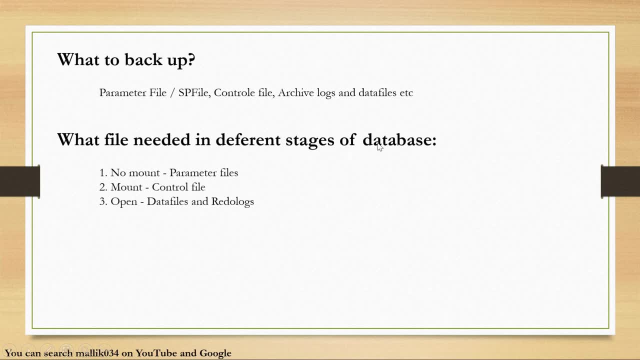 So needed in different stages of database? like database, different stages are like no mount, mount and open. And what are the files are needed? In no mount, we need parameter file or SP file. In mount mode we need control file And in open mode we need a data file or a read to log file. 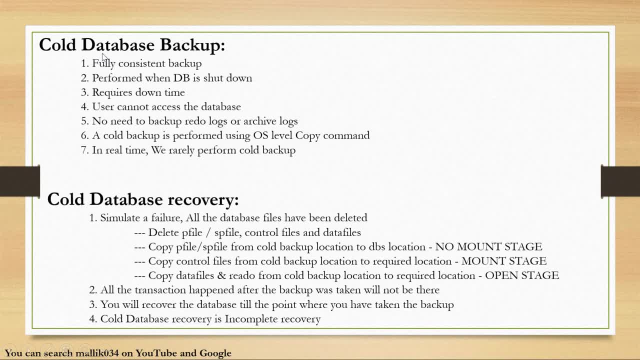 Okay. So the cold backup and cold recovery, Cold database backup and cold database recovery How it works: Fully consistent backup. Cold backup is a fully consistent backup Because we are setting down database and taking the backup And performed when DB is shut down requires the downtime. User cannot access the database. No need to backup, read to log and archive logs Because you are setting down database. you are just copying your data files and control files. A cold backup is performed using a OS level copy command, CP command- In real time. we rarely, we hardly use this cold backup. Nobody will prefer. But in sometimes we need a cold backup. So this is about the cold backup. 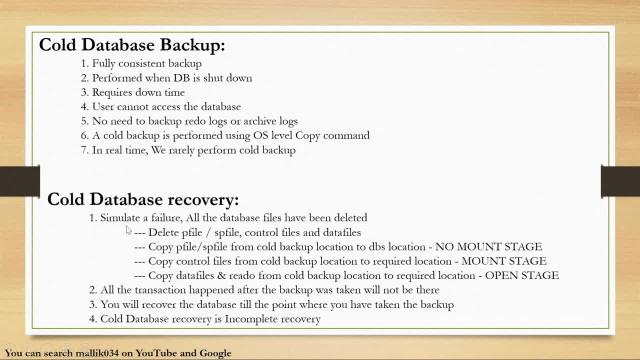 And cold recovery. like how you can do the recovery: Simulate a failure. All the data files have to be deleted. Like you know, you can delete all the data files from the location And then delete, like how you delete. Delete P file or SP file and control file and data file And copy your P file or SP file from the cold backup to the DBS location And then you, you know, start your database in no mount Because you got your P file. 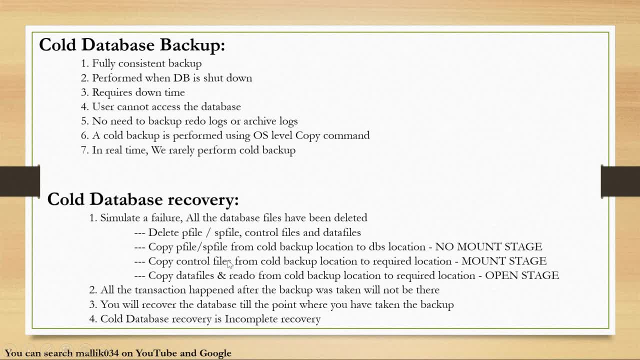 Copy your control file to the wherever location it is pointed in SP file And then start your database in mount stage. So you know, using this backup control file you can able to mount your database And copy your all data files and read to log files to the desired location And then open your database So this time you can recover it. in case of you have a cold backup, All transactions happened after the backup was taken will not be able to, will not be there Because it's inconsistent. you know backup. 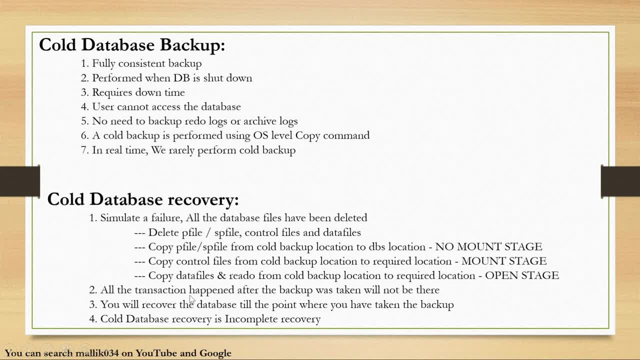 It will not be having entire backup. It is inconsistent recovery right. So it is not behaving any transactions after the backup. You will recover the database till the point where you have taken your backup. The cold backup is a cold. cold database recovery is a incomplete recovery. It is incomplete recovery right. 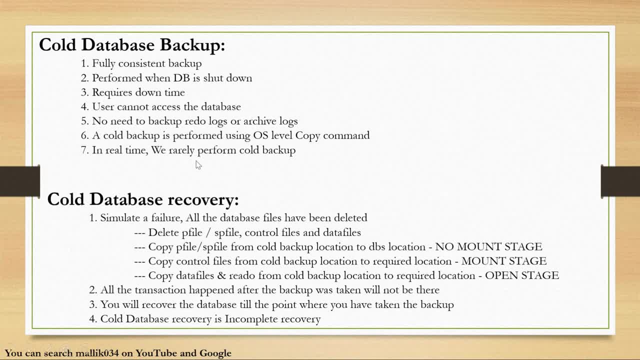 So, because you were going to restore it until you know what time you were taken back. If you taken cold backup on Monday, So you will be able to restore till Monday, And if you, if you lost your data files on Tuesday, 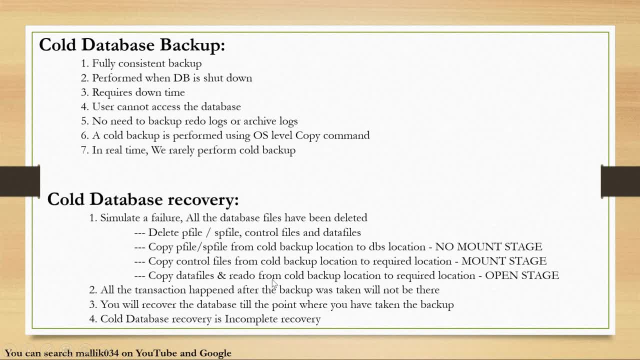 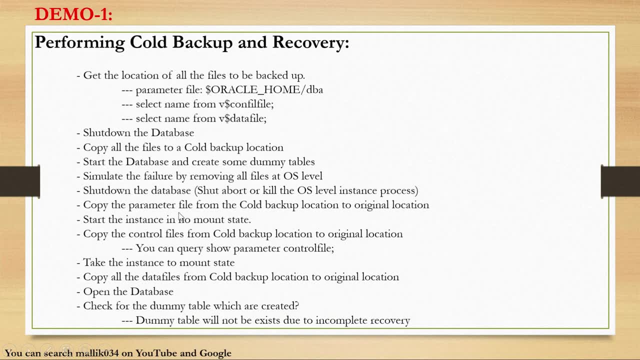 so monday to tuesday so that data will not be available. that is called incomplete recovery and the demonstration like uh performing cold backup and recovery. so this demonstration i'm going to show you uh in in next session. um, just a brief you. what are the steps are involving here? 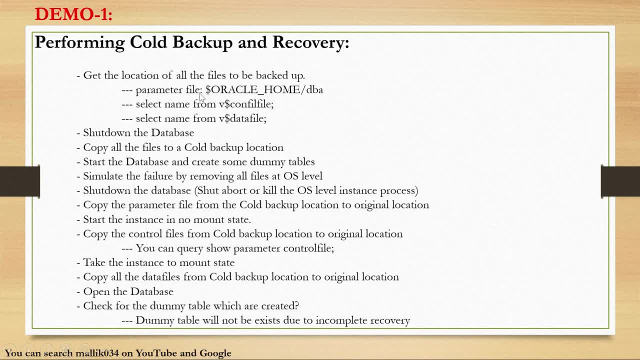 get the location of your uh, all the files- uh parameter files and data control files and data files and shut down your database. copy all this file to a cold backup location and start your database and create some dummy tables and simulate failure by removing all your os level files. 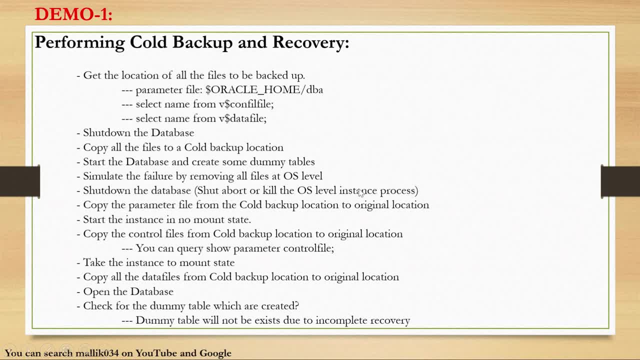 and shut down your database and by using shutdown, abort or kill your os process and copy parameter files from cold backup to original location and then start your database in no more state and then copy your control file from the cold backup location to original location and you can. 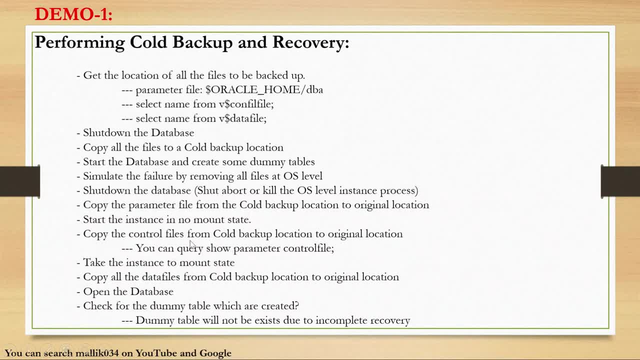 uh, you know you can get the control for location in in your pfi and then start your you can. you know you can take your instant with me mount state and then copy all your data files and read aloud files. uh, from the cold backup location location to the original location and you can open your database. uh, check for the dummy table. 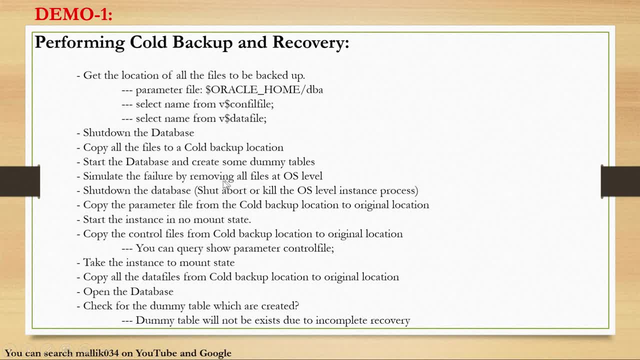 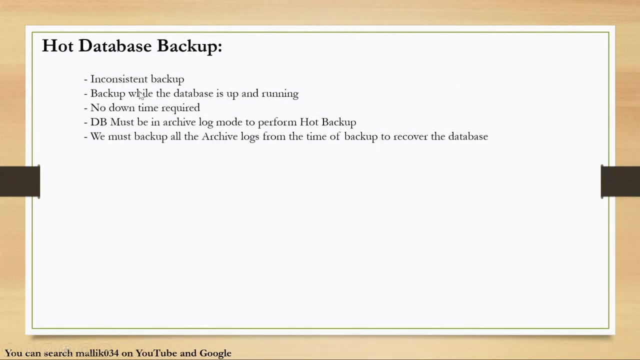 which you created uh before the uh simulation of this crash or no deletion of this file dummy table will not be exist because it's incomplete recovery. so this dummy table created after my backup. so, coming to the hot backup: hot cup, hot backups are inconsistent backup. backup, uh, you know, performed while a database is up and running and no downtime is required. uh for this. 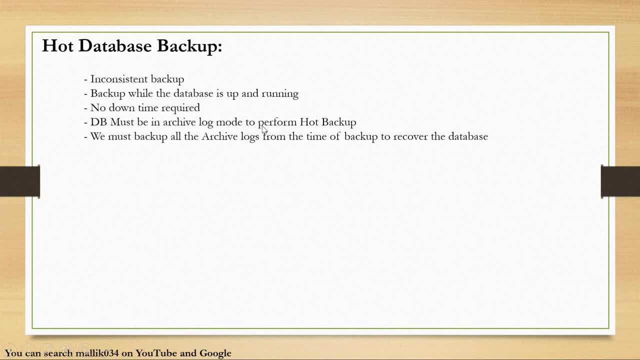 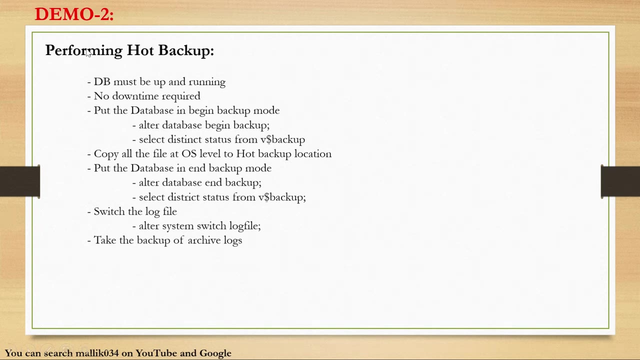 hot backup and db must be in arca log mode to perform this hot backup. and we must, uh, you know, backup all the archive logs, uh, from the time of backup to the recovery database. all right, this is about the hot backup, and the demonstration for hot backup is performing hot backup. db must. 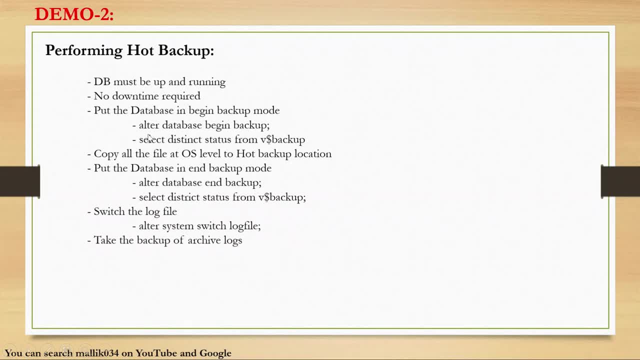 be up and running, no downtime required. put database in begin backup mode. alter database: begin backup. select distinct status from v$backup. check that status of your backup and copy all your- you know- OS level files to hot backup location. and whatever your backup location, you just copy it and put database in end backup mode, like alter. 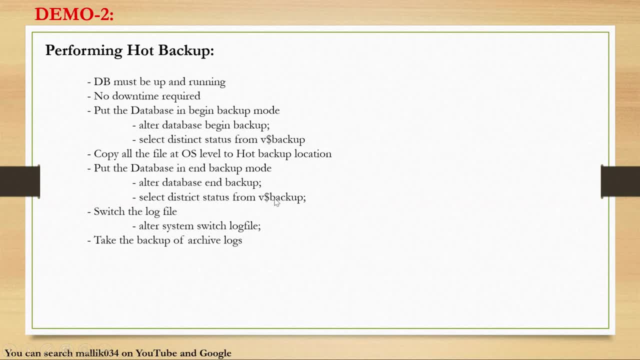 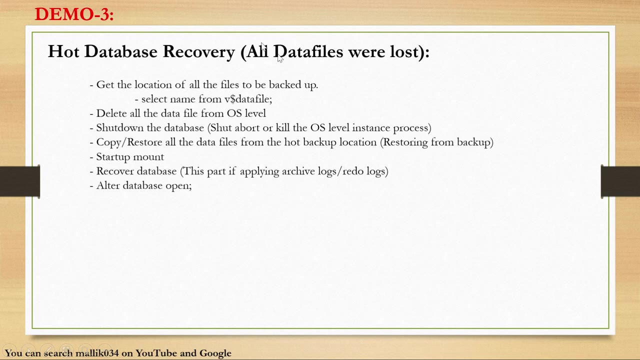 database, end backup and select distinct status from v$backup. it will show that backup completed and then switch some ArcaLogs. alter system, switch ArcaLogs and take ArcaLog backups. so this is about performing your hot backup and hot backup recovery. when you lost your all data files, assume that you lost your all. data files and you have taken hot backup, and then how you can restore it. get a location of all your files to be backed up, like select name from v$data files, and delete all files from OS level. you can delete it and then shut down your database or shut down about or kill your OS process and then you will not be. 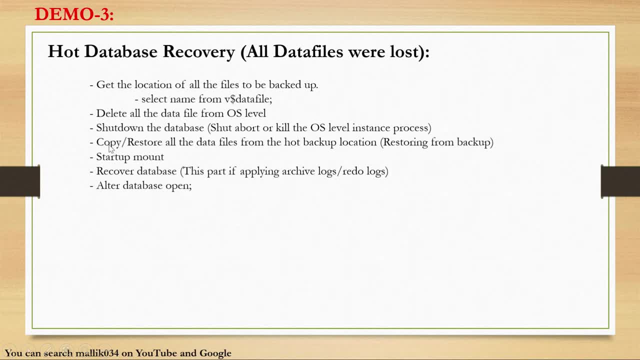 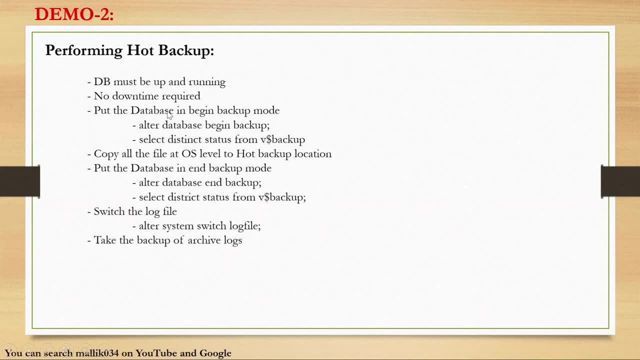 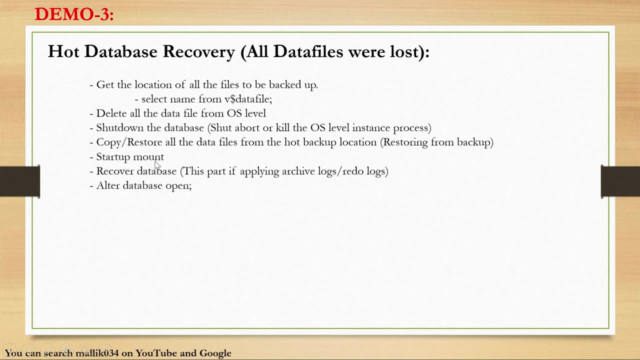 able to start your instance back so that you know, doing that time you can copy, restore all data files from hot backup location, whatever you were taken from the previous hot backup, to the the backup location and then start your startup mount, start your database in mount mode because you 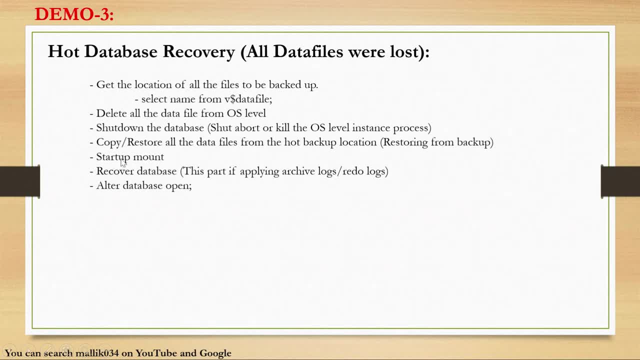 already have your p file and you have your control file, you can directly mount your database and recover database. this will apply all your ArcaLogs and read logs and then alter database open. this is about you know if you are having hot backup, how to recover your database. 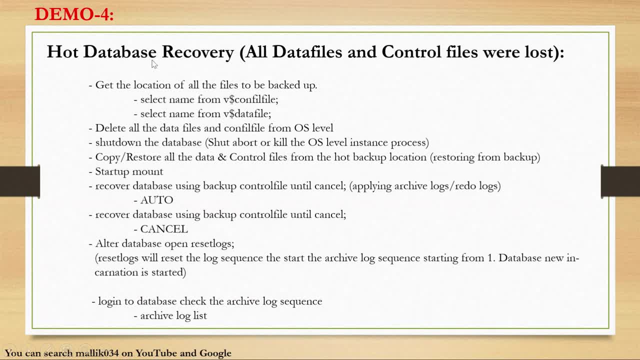 and then hot database recovery in case of all data files and control files were lost. so that time how we'll do get your location of all the files to be backed up like name. select name from v$control file. select name from v$data file. delete all your files and control files at the OS level and shut. 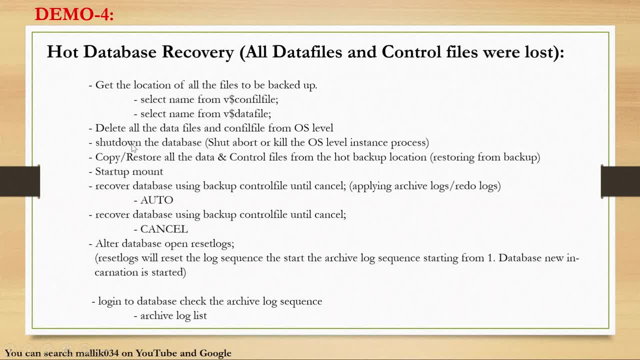 down your database like shut about or kill your OS process and copy or restore all your data files and control files from hot backup location to the original location and start up mount and recover database using backup control file until cancel. it will apply all your archive log and re-log like either auto or cancel. 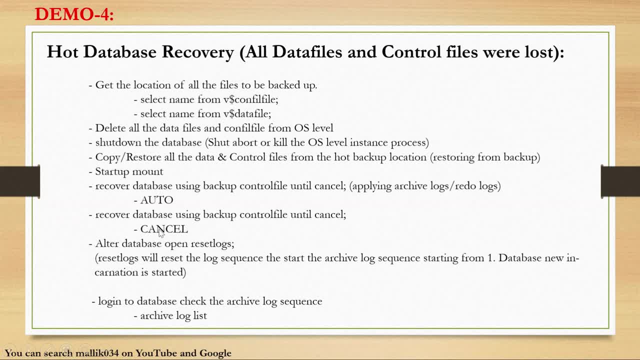 recover database using backup control file until cancel and then you need to cancel at certain point after applying all the archive logs and then alter database. open reset logs and reset log will reset log sequence and start archive log sequence starting from 1 and database new incursion is started and login to database. 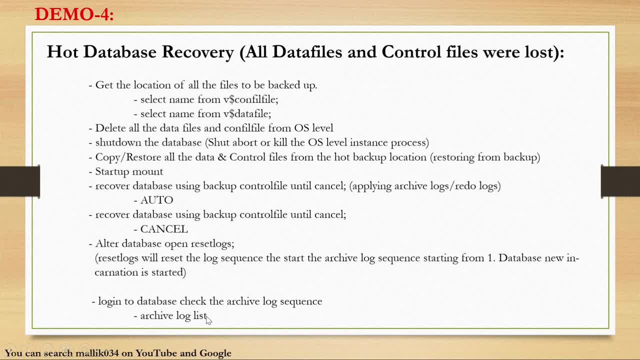 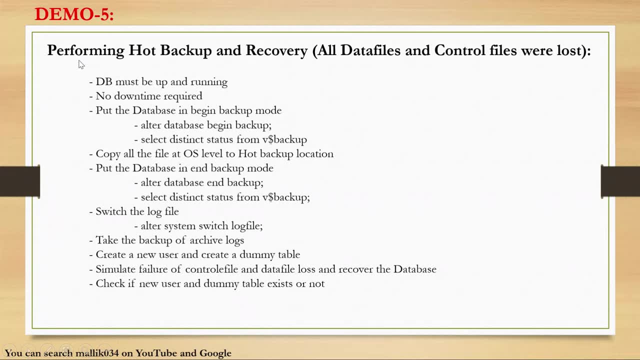 and check archive log sequence. archive log list will be started with sequence number 1. this is about when you lost your control file and data files, and demo 5 talks about performing hot backup and recovery. all data files and control files were lost. this is same as demo 4, but here in this demo 5. 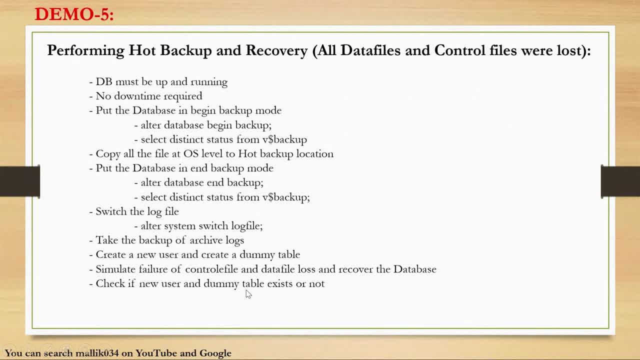 i am going to create some dummy tables and you know whether i will be able to check those dummy tables or not. this is about some transactions you know performed after the backup. what i am going to do: db must be up and running. no downtime record. put your database in begin backup mode. alter database: begin backup alter. 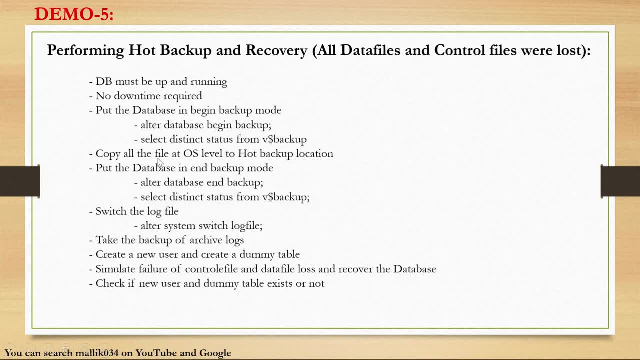 select distinct status for middle or backup and copy all the files at the os level to your hot backup location and put database in end backup mode. alter database end backup and select distinct status for middle or backup. it says that backup completed and switch some archive logs and. 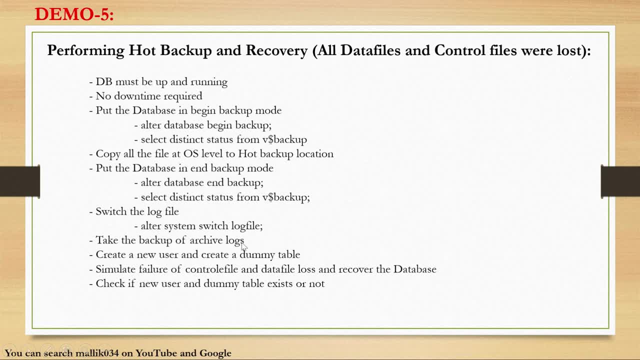 alter system, switch archive log file and take a backup of all your archive logs and create a new user and create some dummy tables and simulate the failure of control file and data files and now recover the database. so whatever you did here, like deleting all these files and recovering, and you do it here. 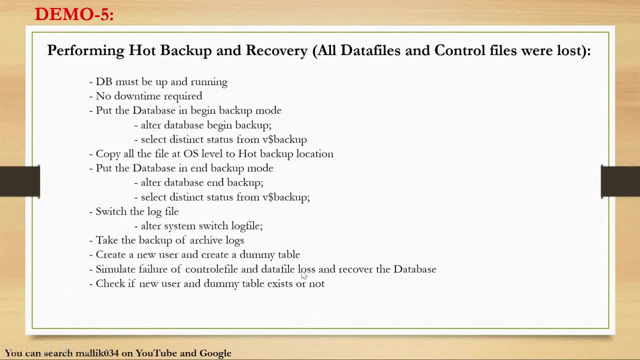 everything. same step like this. this step will talk about the same, the demo 4, what we did- and check if the new user created after the backup and new dummy table created after the backup is available or not. if you see here, you are going to create new user after the backup, so after recovery, whether you are able to see this. 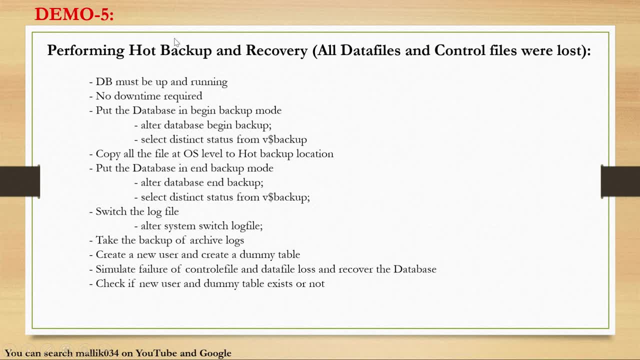 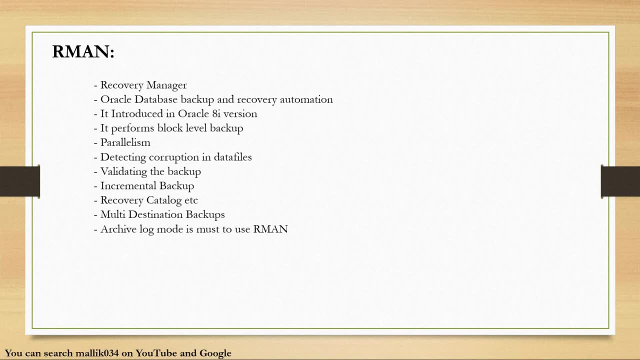 or not. we are going to show, we are going to check it out. this is about demo 5 and coming to the RMAN recovery manager. RMAN stands for recovery manager, oracle database backup and recovery automation. this is the. this is the one of the widely used tool most of the industries. 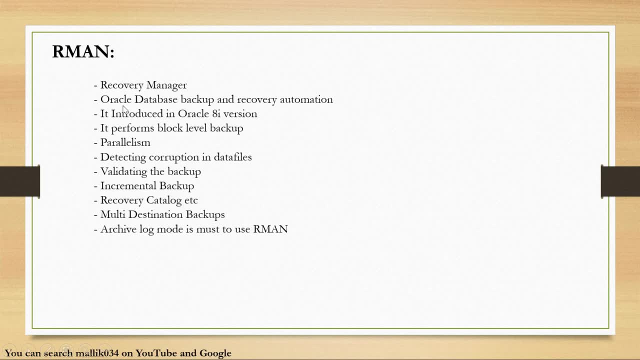 are using RMAN as a backup and recovery tool and it is it has introduced in oracle 8.8i 8i version. it performs the block level backups and it supports for the parallelism. you can have a parallel threads for the backup for the. 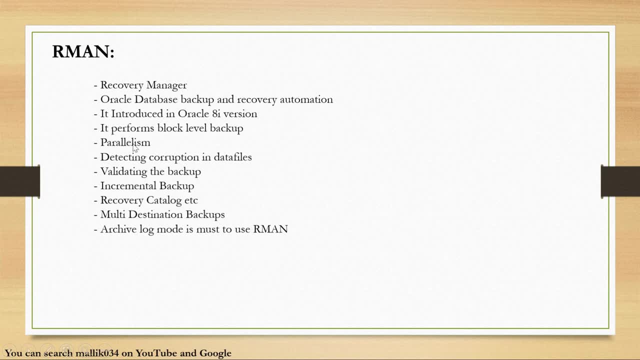 similarly for the restore also. you can use this RMAN and you can use this parallelism for the recovery and detect, detecting the detection of the corruption in data file. you know it can detect corruption in data file. validate the backup after you perform RMAN backup or you can validate your backup. 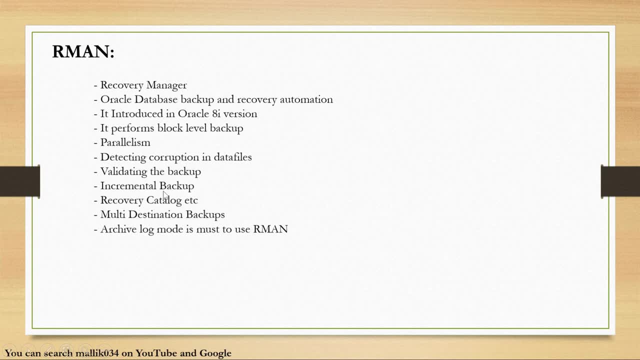 whether it's a consistent or whether it's a valid backup or not, and you can take an incremental backup and you can have a recovery catalog to have your backup information and it's a multi-dimensional backup. archelog mode is a must when you use RMAN. 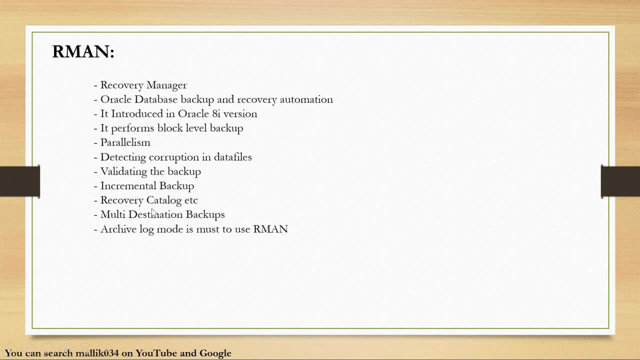 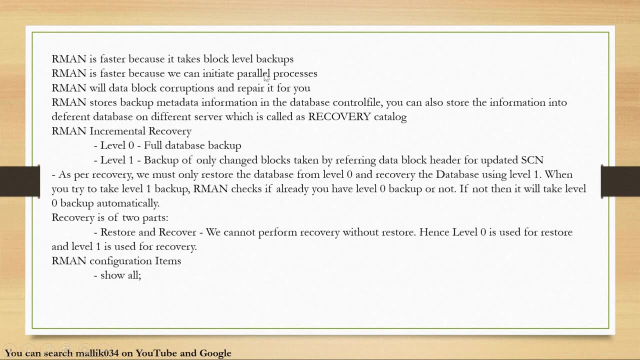 these are the characteristics of RMAN, and RMAN is the faster because it takes a block level backup. RMAN is faster because we can initiate a parallel resource. RMAN will do a block corruption and repair it for you. like you know, it will check for any block corruption and then it will automatically try to. 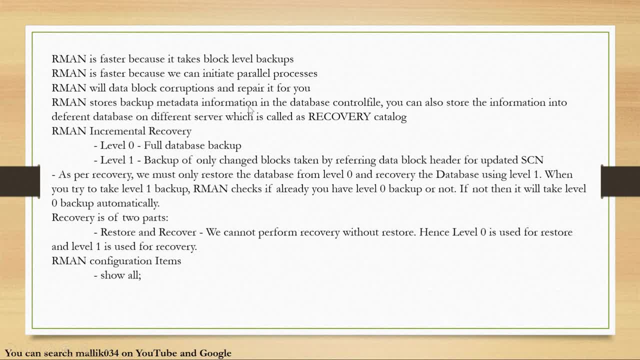 repair that block corruption. RMAN stores backup metadata information in the database control file. you can also store the information into a different database on the different server, which is called a recovery catalog. you can have either recovery catalog or you can have your backup information in your control file. RMAN incremental backup like. 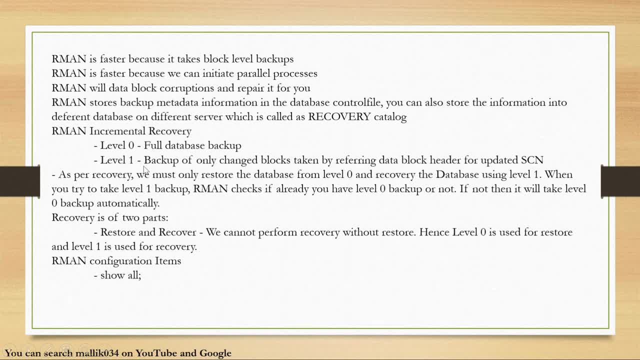 level 0 and level 1. level 0 is a full database backup and level 1 is a backup of only changed blocks taken by referring data blocks header for the updated SCN. whatever the changes after level 0, only those changed backup will be performed in level 1 and then. 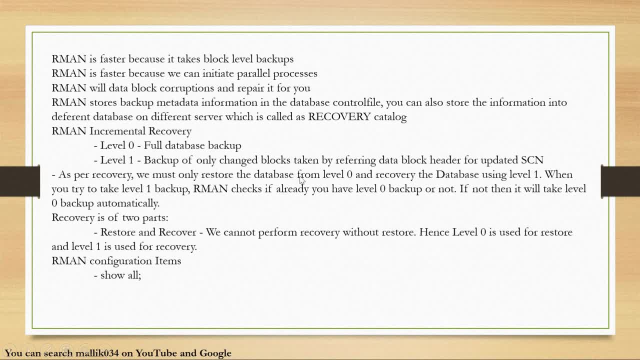 as per recovery, we must only restore the database from level 0. we are going to restore from the level 0 and recovery the database using level 1. using this level 1, we are going to recover it. when you try to take a level 1 backup, RMAN checks if already level 0. 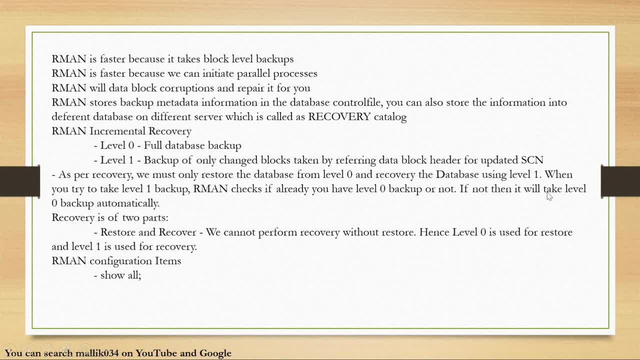 backup is available or not. if not, then it will take a level 0 backup automatically. this is one of the point, like if you don't take level 0 backup and directly start level 1 backup and it will check for level 0. if level 0 is not there, it will start level 0 automatically. 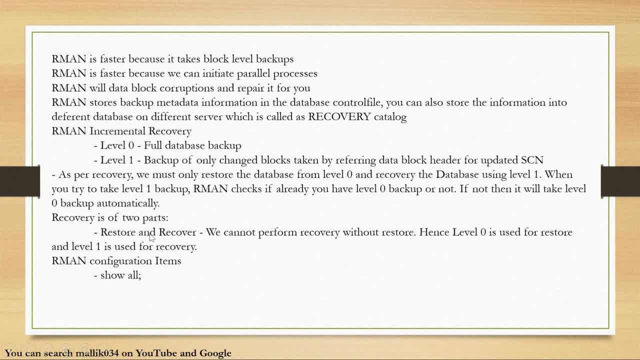 the recovery is having two parts. one is restore and recover. we cannot perform recovery without restore. hence level 0 is used for restore and level 1 is used for recovery. RMAN: is you know RMAN configuration items? if you, if you show like show all, it will show all your RMAN configuration. 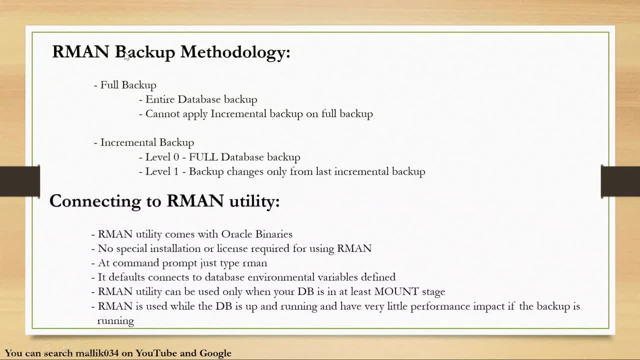 and RMAN settings and coming to the RMAN backup methodologies, like full backup and incremental backup. like full backup, entire database backup. cannot apply incremental backup on full backup. if you take a full backup, it is kind of entire database backup but you cannot apply any incremental backup. 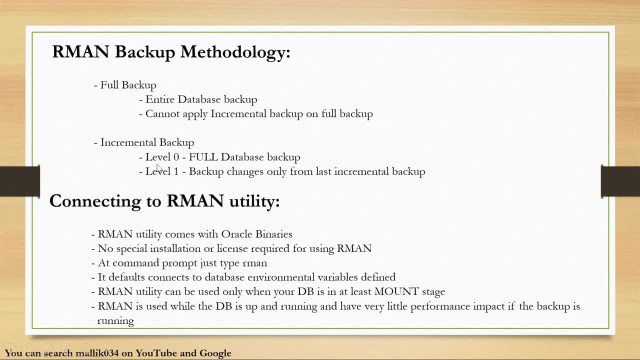 on full backup. but coming to the incremental backup, it has level 0 and level 1 backup. level 0 is same as your full database backup and on top of this level 0 you can have your incremental backup level 1 backup. level 1 backup is nothing but backup, changes only from the last. 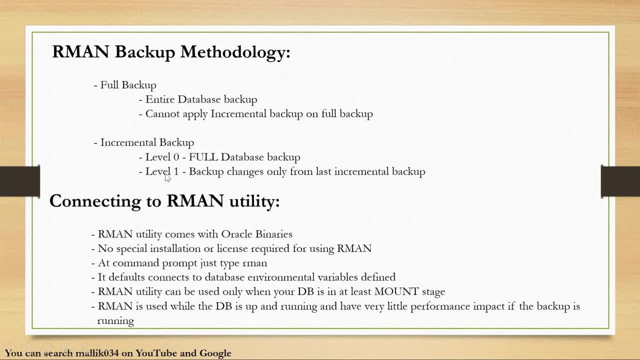 incremental level 0 backup and again in level 1 we will be having cumulative backup and differential backup, so that I am going to cover later. and connecting to the RMAN utility. RMAN utility comes along with Oracle binaries. whenever you install your binary, RMAN will be installed, no special 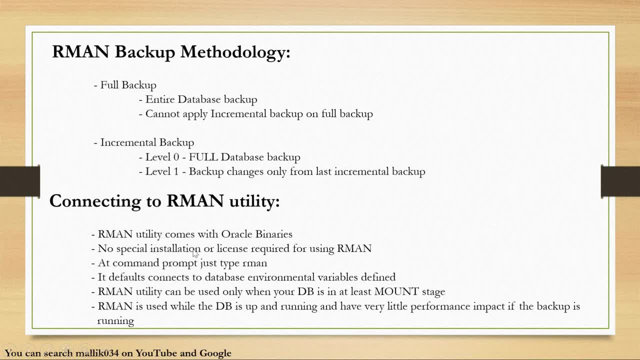 installation or license required when you are using RMAN because it comes along with your binaries. at a command prompt you just type RMAN and then it will go to RMAN command prompt. it default connects to database enrollment variable defined like whenever, whatever the enrollment variable is set. 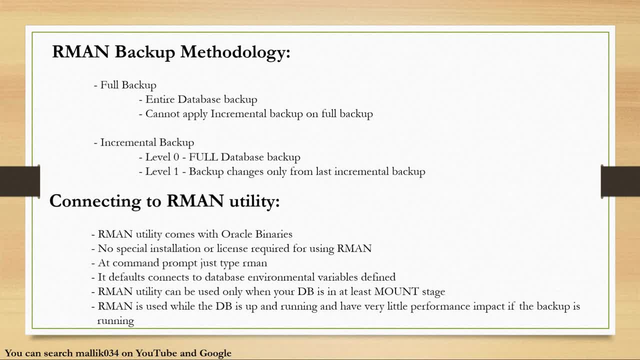 so it will default connect to that enrollment and until unless if you don't specify the RMAN target, RMAN utility can be used only when your DB is in at least mount stage. so if it is in no mount stage you cannot use RMAN. RMAN is used. 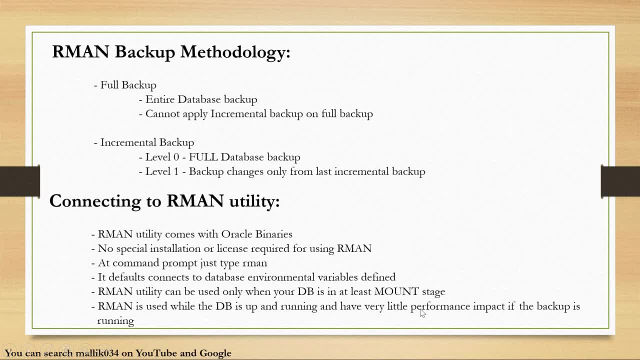 while DB is up and running and have very, very little performance impact when you have backup is running. so one of the best tool, RMAN. like when your RMAN backup is running so you won't see any performance issue at the database level- actually slight, slight impact. but whereas when you are, 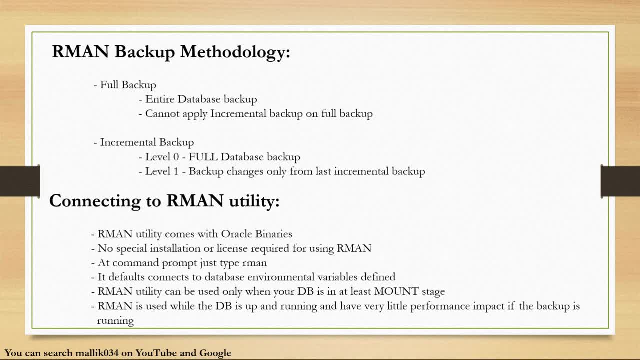 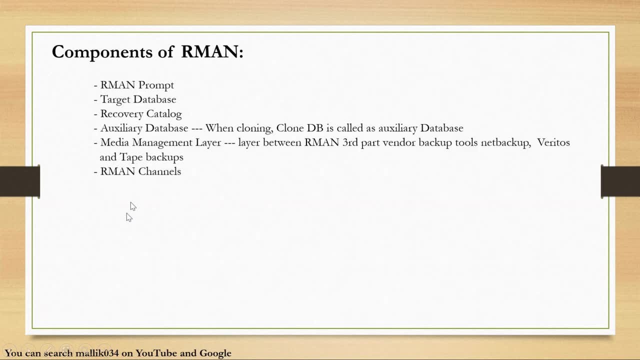 having a hot backup when you're keeping your database in begin backup mode there might be, you know there is a huge performance impact. that's one of the major advantages of having RMAN and components of RMAN like RMAN prompt target database and recovery catalog. like RMAN prompt is same as your ksql prompt. 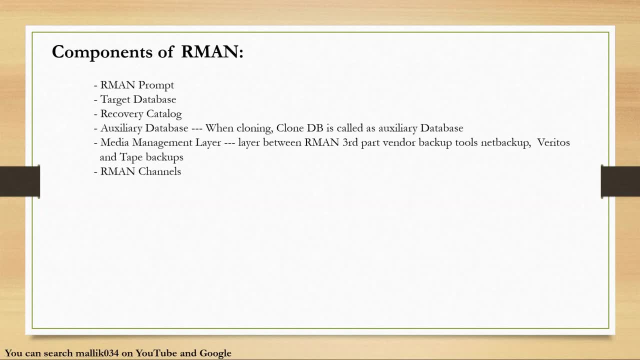 whenever you connect RMAN it will connect to its own RMAN prompt and target database. you have to define your target database so that you know it will directly connect to target database and recovery catalog to have your RMAN backup information and auxiliary database when cloning- clone DB. 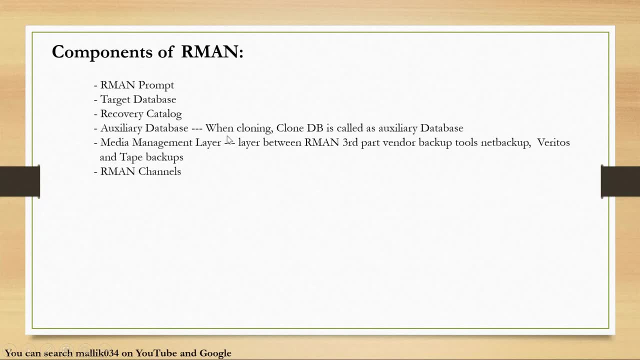 is called auxiliary database when you are cloning your, you know, lower database, like test database or a dev database, or when you are restoring your secondary database data guard. so all your target database is called as auxiliary database and media management layer between RMAN and third party vendor backup tools. 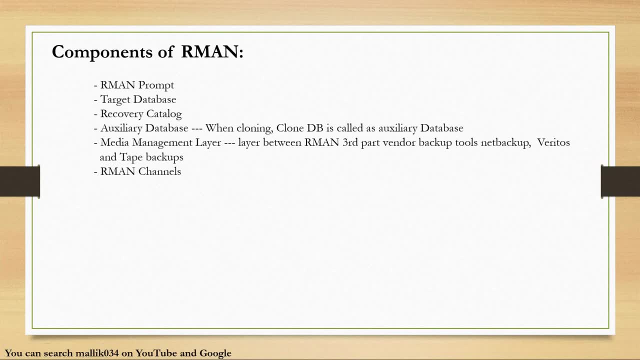 like net backup or veritas or trivoli or any any backup. the media layer between the RMAN and then the third party vendor backup tool is called media management layer, and and also between the tape backups like and then other characteristics are like RMAN channels. you can define a number of channels. 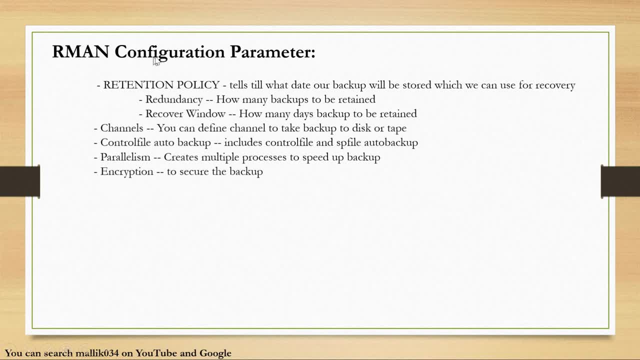 for your backup and recovery and RMAN configuration parameter, like retention policy, tells till what date your backup will be restored. which can we use for recovery. you know retention policy will be redundancy. you know recovery window. redundancy is how many backup copies you can retain and redundancy window means, like how many days you 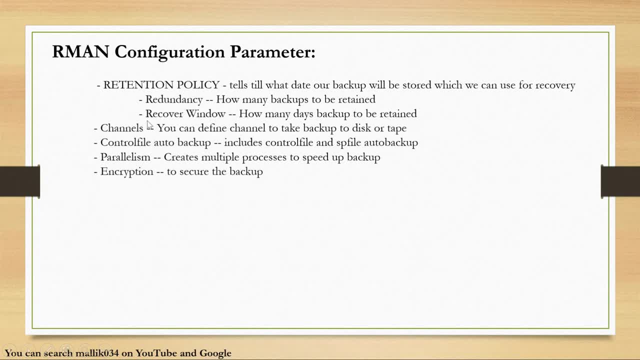 can backup to be retained right, like, for example, seven days. if i mention so up to seven days, my backups are valid and then i can use it for recovery. redundancy means redundancy, seven means up to seven backups. i can keep it for recovery and those are all valid and those seven backup copies can be used for. 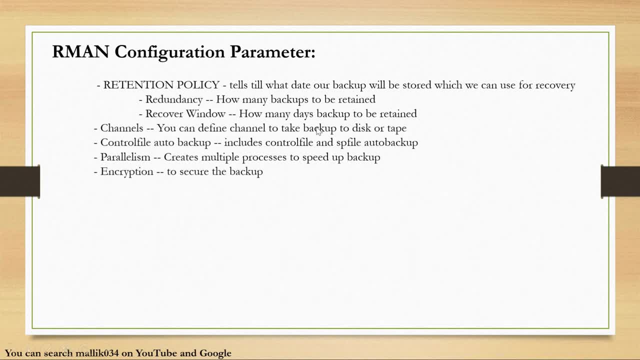 recovery and channels. you can define channels to take a backup for the parallelism like you can. you can define four, eight, ten, whatever channels your OS supports you can define for restore and recovery. control file, auto backup includes control file and SP file. auto backup and parallelism creates multiple process to speed. 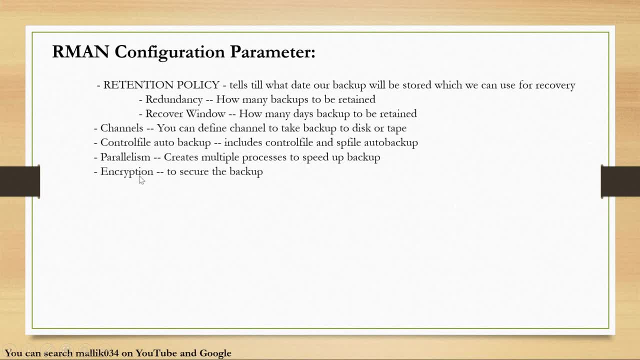 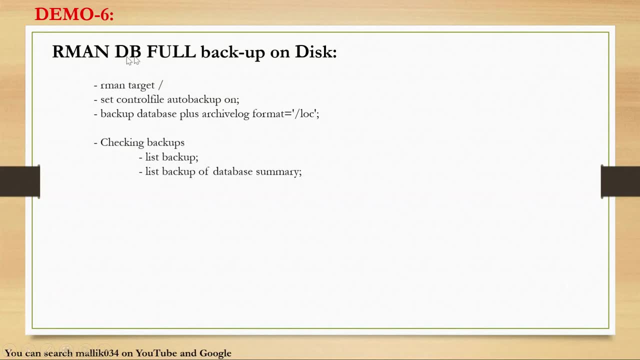 up backup and as well as recovery. the encryption is the secure backup. you can have your backup encrypted and demo. six talks about RMAN db: full backup on the disk. like you know, just need to connect RMAN target slash. it will connect your target database and set control file auto backup on and then backup database. 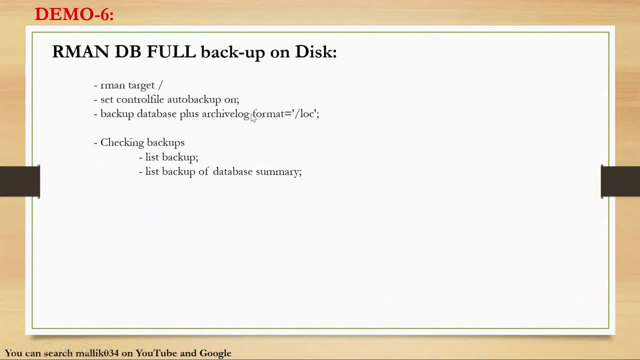 plus archive log format. you can give any location. it will take your full database backup plus archive log and check the backups. like in the RMAN prompt you can do list backup. it will show what is your backup and where is your backup, and list backup for database summary it will give you. 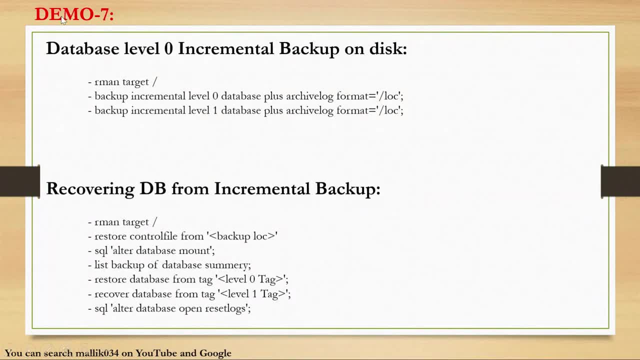 entire summary of your backup and demo. seven talks about database level zero: incremental backup on disk. like connect to RMAN, like RMAN target slash backup. incremental level zero database plus archive log format. you can give any disk location and whereas level similarly to level one backup incremental level one database. 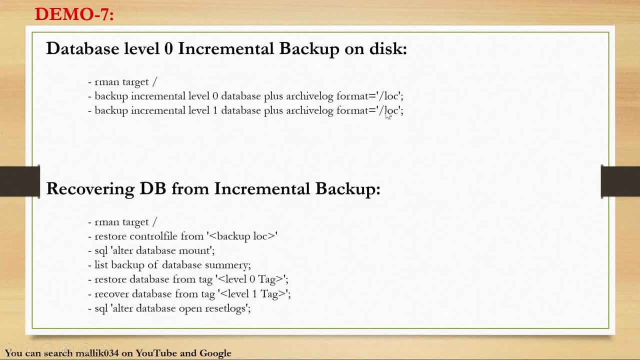 plus archive, log and format. you can give any database location, any OS location. it will take. this is level and level one: backup and recovery. db from incremental backup. connect to RMAN target slash. restore your control file from backup location. wherever you have taken your backup, you have to mention that backup location and sql alter.